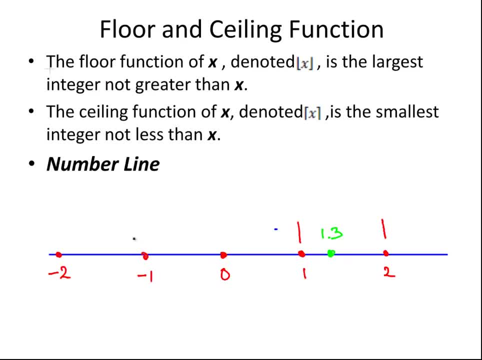 So ok, Now let's go to the other end here. Let's suppose we are dealing with minus 1.5. let's say Now, this is be very careful here, And it's actually a good idea to visualize the number line when you are doing these. 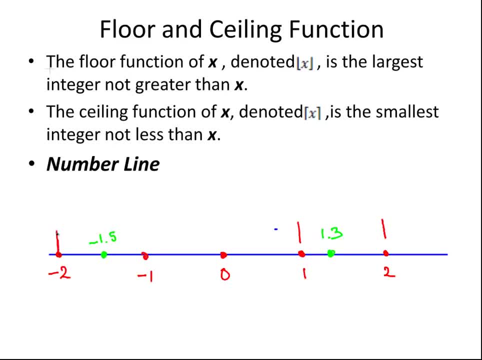 The integer that precedes it in the number line is minus 2.. And the integer that comes after it is Is minus 1.. So that could be a bit very counter intuitive. So let's write that out: The floor function of 1.5 is minus 2.. 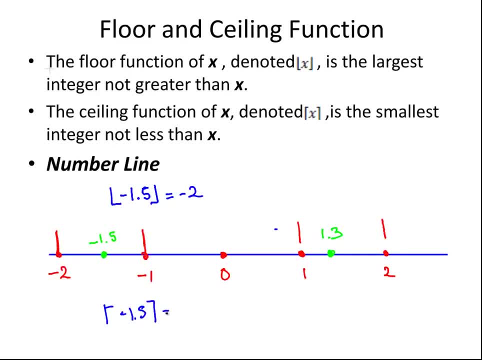 The ceiling function of minus 1.5 is minus 1.. Likewise over here, the floor function of 1.3 is simply 1.. The ceiling function of 1.3 is 2.. It's actually usually on the negative side of the number line. 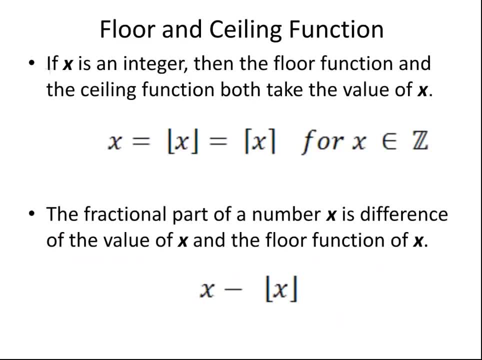 That we run Into problems. Ok Now, if x is an integer, Then the floor function and the ceiling function both take the value of x. So if x is an integer, x equals the floor function of x equals the ceiling function of x. 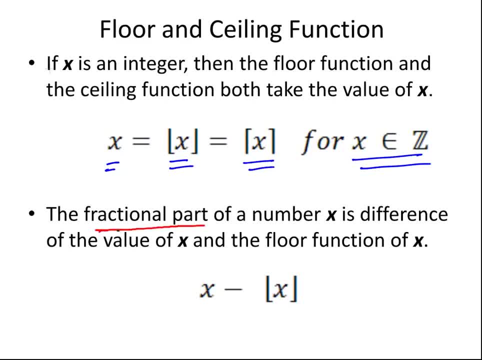 Now a useful sort of Another extra sort of component that is brought into consideration When we are doing these type of problems Is the fractional part of a number x. It's the difference of the value of x And the floor function. So we write it like this: 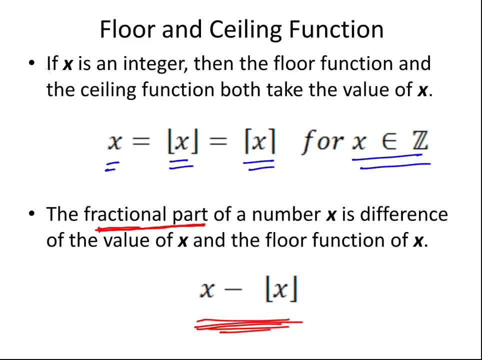 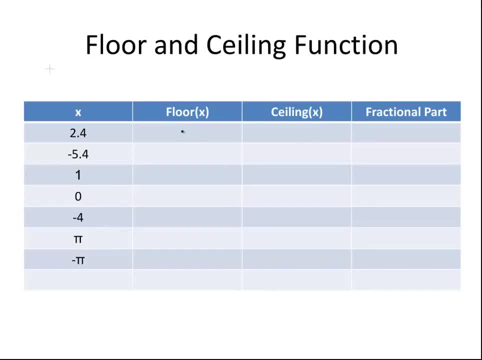 x minus the floor function of x. Ok, Let's look at some examples here. So 2.4.. Floor function of that Is 2. The ceiling, 3. And the fractional part, 2.4 minus 2.. 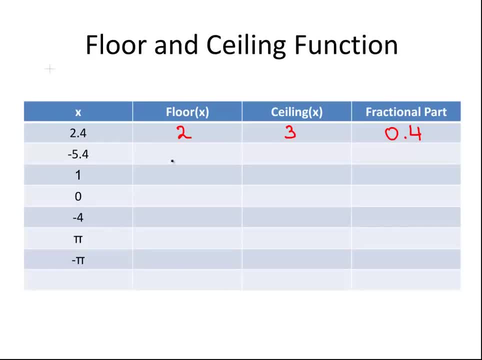 That is 0.4.. The floor function of minus 5.4.. Just remember the number line. It's minus Minus 6. And in this case the ceiling is minus 5.. Now Let's do the fractional component here again. 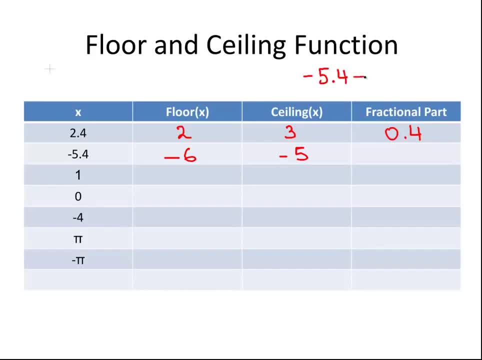 You might be surprised by this result: Minus 5.4.. Minus, Minus 6. The minuses cancel out. So actually, what we are left with is Plus 6, essentially. Let's just rub that out there.